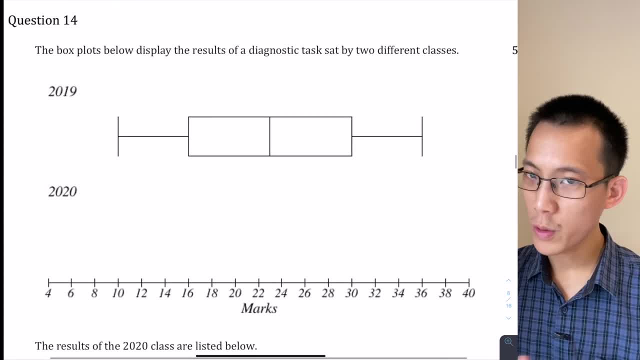 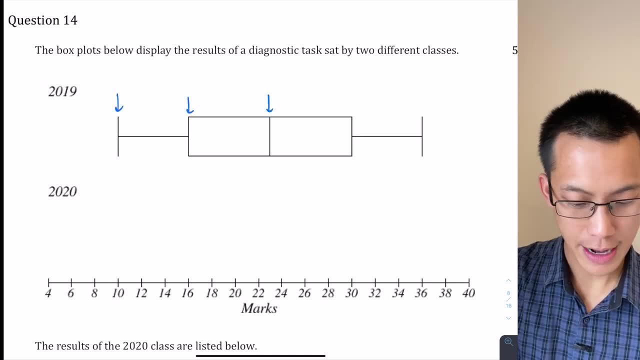 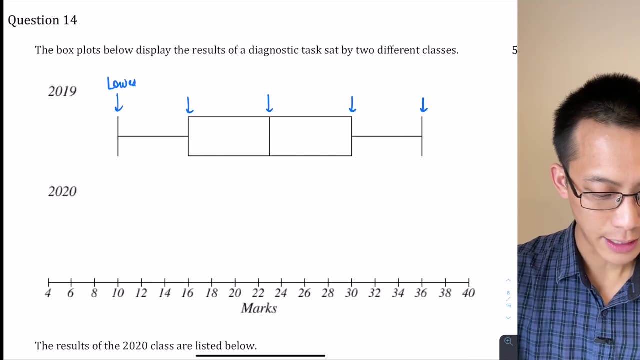 create the box plot. Now you need to remember what does a box plot actually tell you? Well, there's five important spots on a box plot: One, two, three, four, five. If we go from in order, you've got the lowest score down here. And if you have a look at the horizontal axis here for the 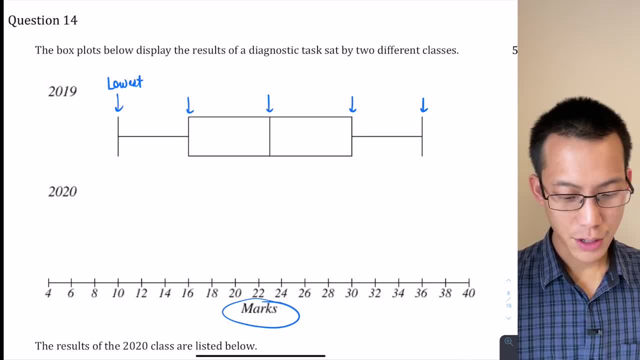 marks. you can see they go from lowest to highest. So there's the lowest score, actually, maybe going all the way to the other end. You can see that implies here's the highest score over on the right-hand side, And then you've got the lowest score on the left-hand side, And then you've got. 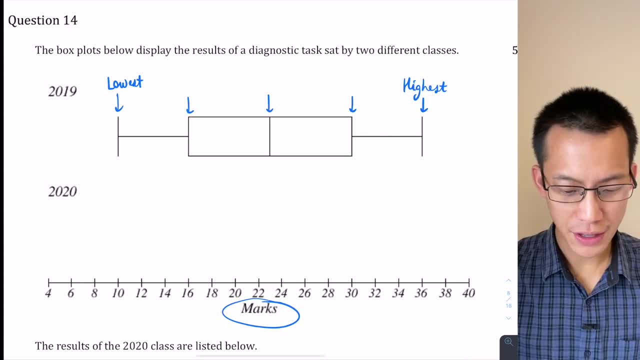 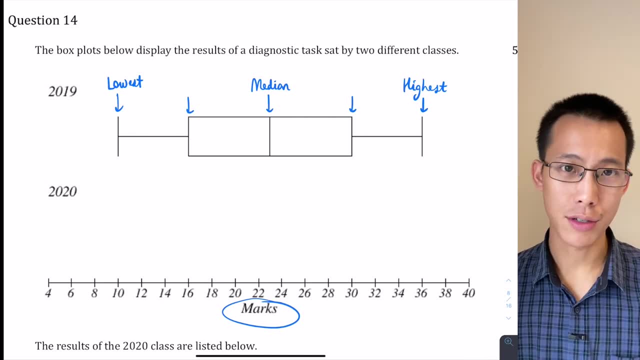 the lowest score on the right-hand side, And then you've got the lowest score on the left-hand side, Right there in the middle. as we've seen before, this is the median, So it's not the mean or the mode, It's the middle score here, the median, And that just leaves you on the two. And this is where. 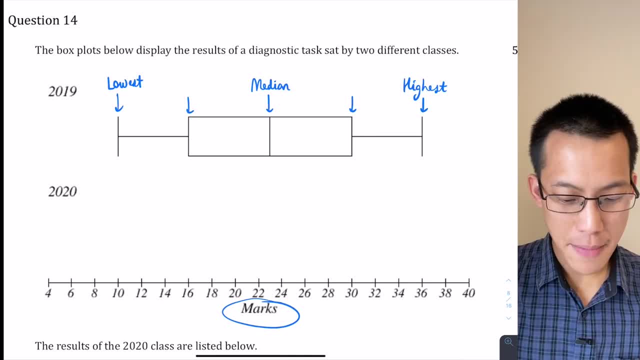 you need to remember what we call our quartiles right Now the median. it breaks up your entire set of scores into two equal sections. So if you had, you know, a hundred students, then the score would break your top 50 and your bottom 50 into two different groups. But these quartiles we call 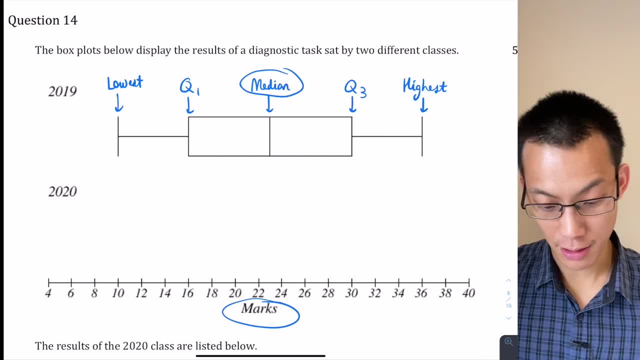 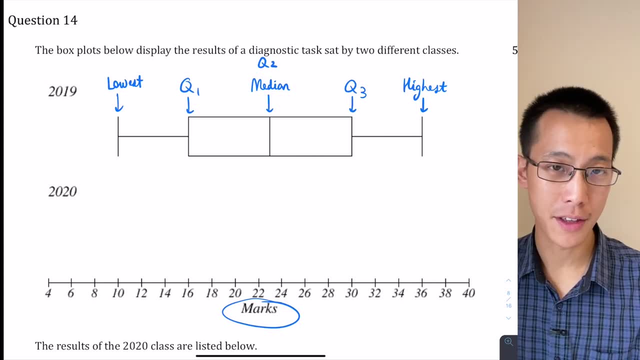 them Q1 and Q3, because the median is Q2.. Q1 and Q3, or Q1, Q2, and Q3 together. they don't break up the data into two. They break the data into four, So that's why we call them quartiles, And you can. 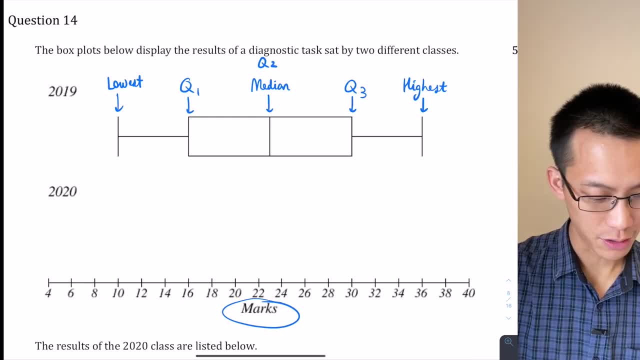 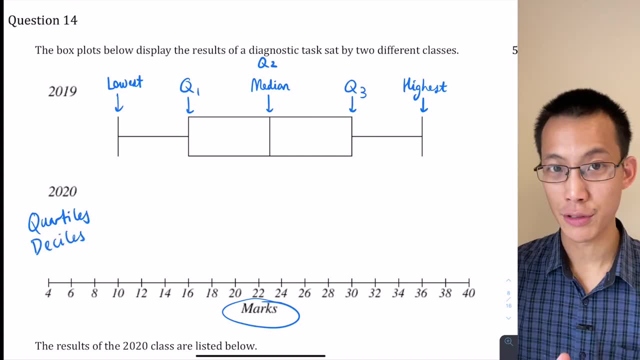 sort of extend this. you know, you've got quartiles- whoops, let's not use an eraser. You've got quartiles which break your data set into four. You've got deciles which break your data set into 10 equal. 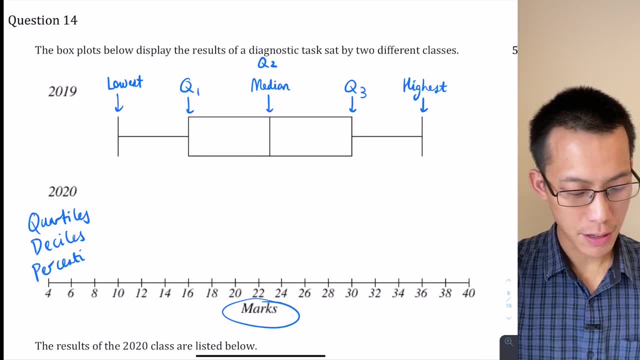 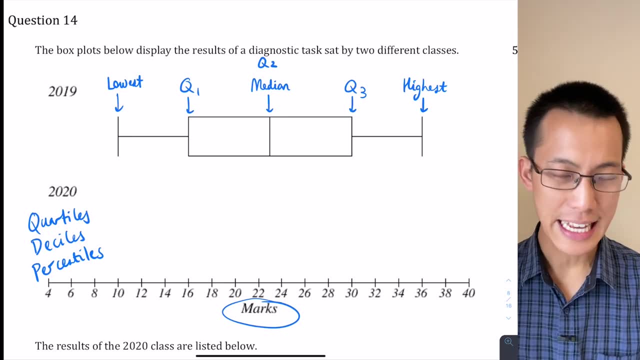 chunks, And then a very common one is the percentiles, which break your data up into 100 different sections, And of course, the most common percentile that people are very familiar with is the ATAR. So people's ATAR tells you, you know, if you've got an ATAR of 75,, that means you're roughly better than 75, or you perform. 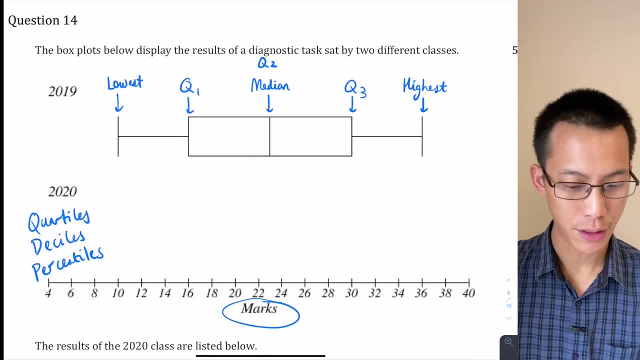 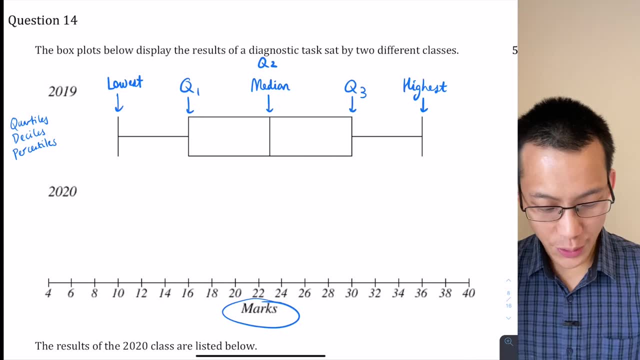 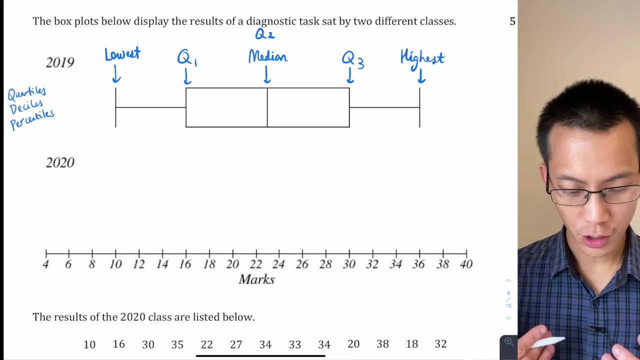 better than 75% of the same cohort who did the exam with you. So we know- let's just push this over to the side here. We know what these data points are supposed to be. How are we going to sort out these data points? Well, what's the ATAR class? Well, because all of these data points here. 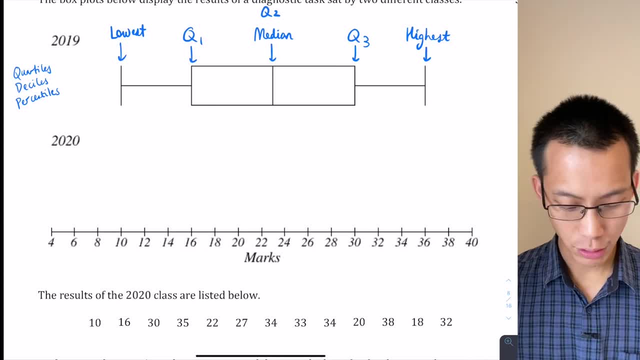 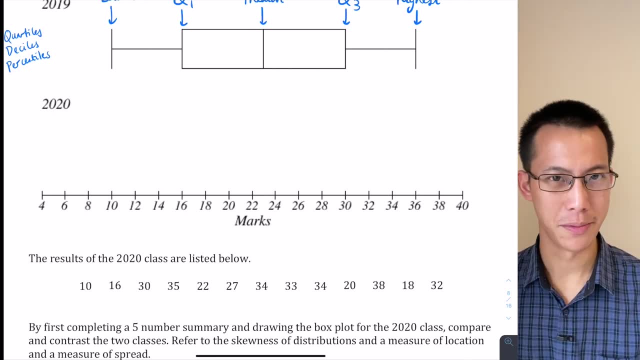 lowest, Q1,, Q2,, Q3, and the highest. they kind of depend on order. So we need to look at this data set here, which is kind of a mishmash of different numbers in random order, Or maybe it's in a different. 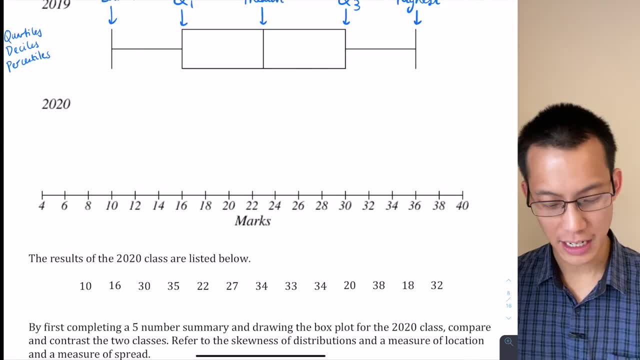 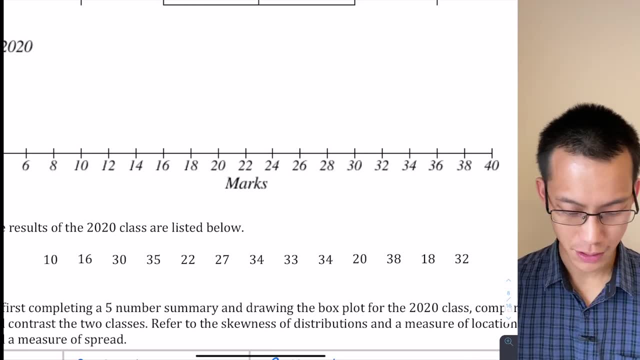 order like, say, alphabetical order, which is not very useful to us, And we need to put it in numerical order And I'm going to say ascending is probably the easiest Now, very practically the way I look here and I don't want to miss any of my scores, So what I'm going to do is I'm going to 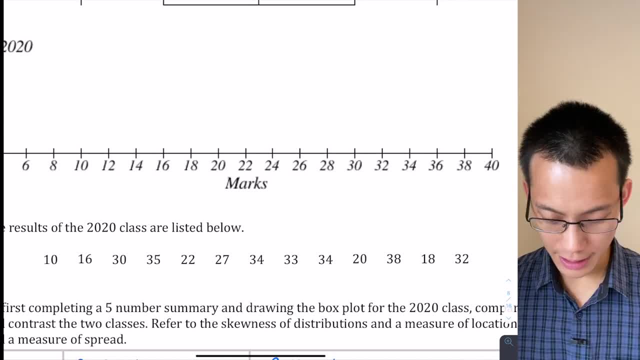 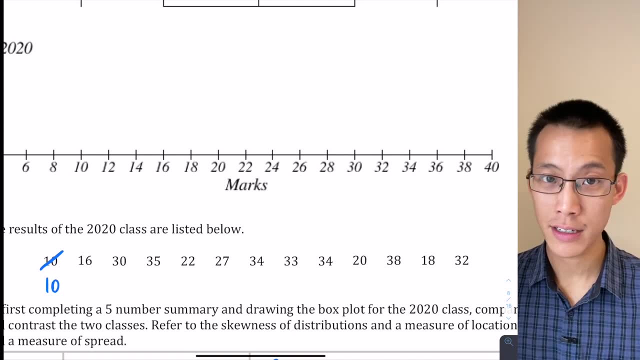 cross off scores as I write them down in order. I look and I see what is the lowest one that I can identify Conveniently. it's actually the 10, which is the first score there, So I'll cross out 10 to. 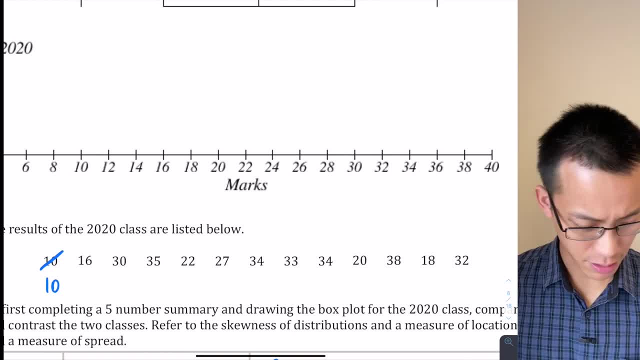 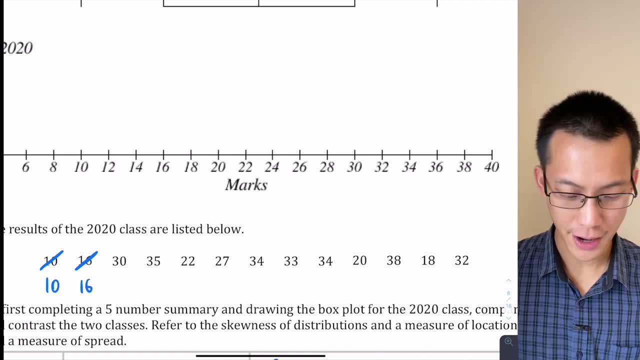 say: okay, this one's done, The next one along again. I'm looking across the entire line Conveniently, it's also 16.. So that's done. But the next highest score is definitely not 30. There's. 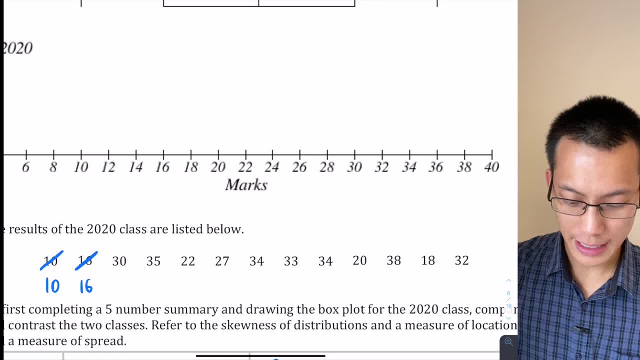 loads of scores that are less than that. So I look and I see across, on the right-hand side it's 18.. So I'm going to write down 18, then I'm going to cross it out. I'm going to keep on going all the. 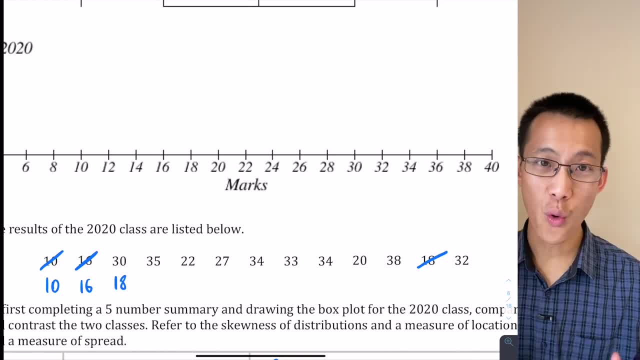 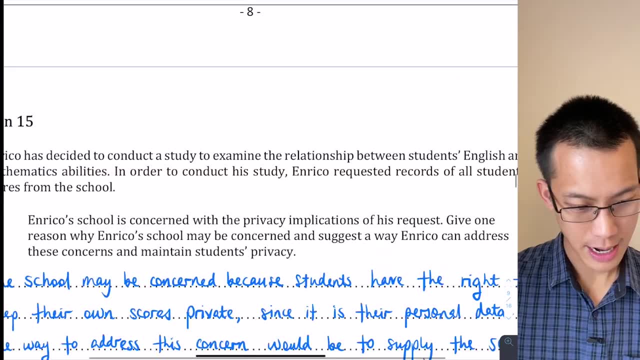 way up, And this way I won't miss any scores, And what I'll end up with is an ordered list of all of the data points. So I'm going to write: let's see here. the next one I can see is 20.. Cross that out. 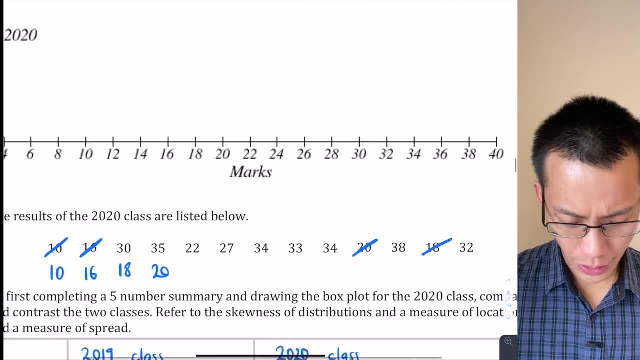 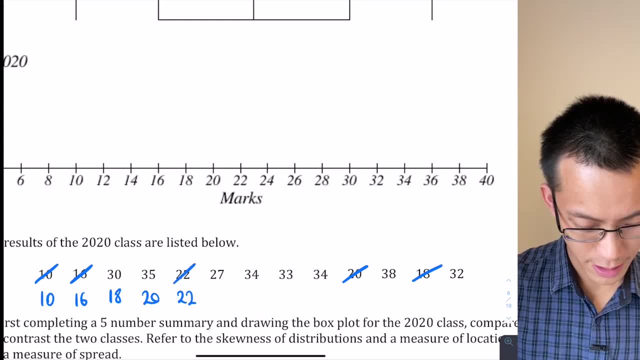 Oops, just go down to the next page by accident. What have we got next here? 27. Oh no, sorry, Missed the 22 there. It's right there. Then the 27. Cross that one out, Next one. by the looks of it, that's the first one in the 30s. Cross out 30.. 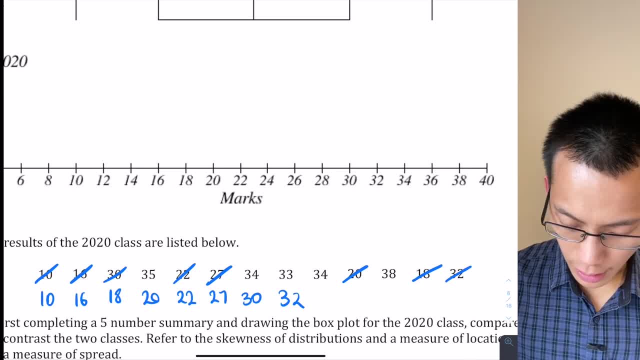 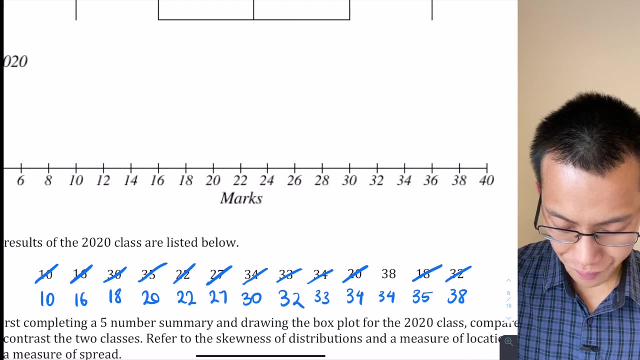 32 is all the way on the right-hand side. 33 comes up, next 34 comes up once, And then it comes up twice. 35 is left over there on the left-hand side, And then the last number is 38.. Okay, 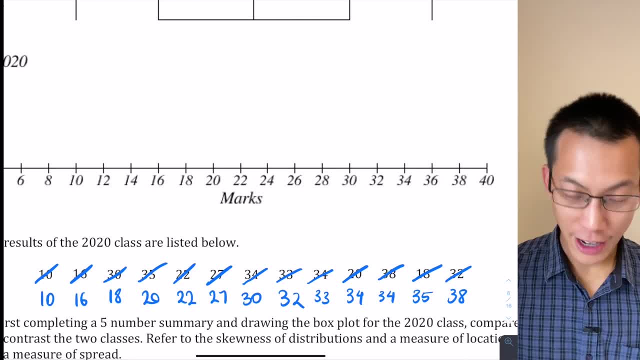 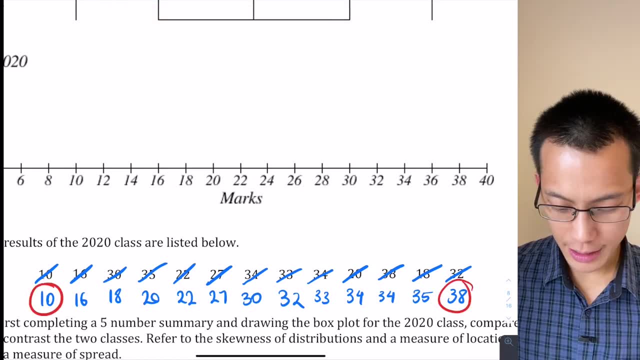 So what have I got here? Well, for starters, I can already read off the first, the lowest score and the highest score immediately. You can see that that's going to be 10 for the lowest and 38 for the highest. So when I go up to my new dot, plot up. 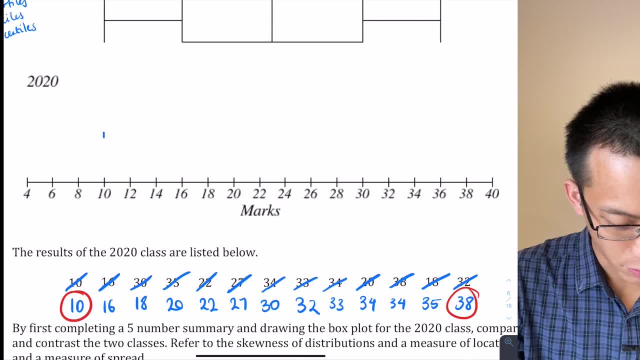 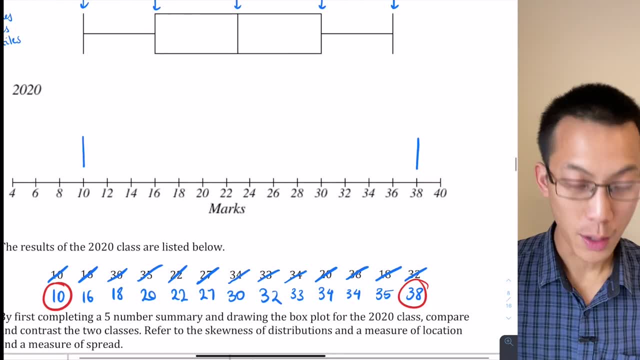 here I'm going to find where 10 is. I'm going to draw a vertical line like so, And then I'm going to go over to 38. And I'm going to draw another vertical line over there. So I've got my bottom. 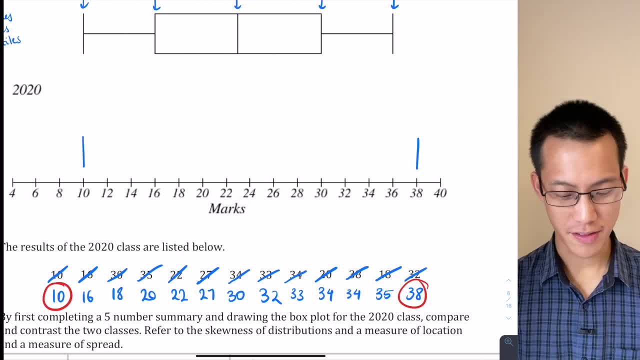 score and my top score. That's good, But now to work out all the rest of them, I need to think a little bit about how I'm going to do this, So remembering that, firstly, the easiest one to find is the median, because it just divides it into half. I need to know how many scores there are in. 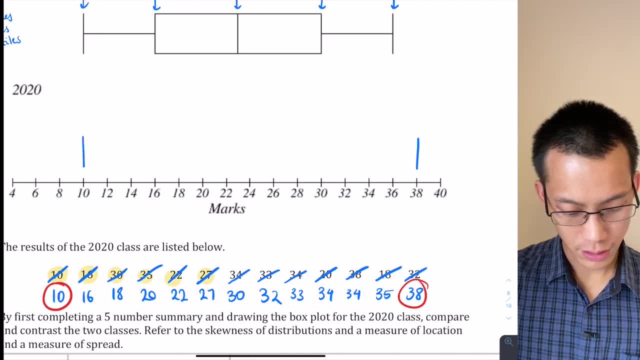 total. So when I go ahead and count, it looks like 1,, 2,, 3,, 4,, 5,, 6,, 7,, 8,, 9,, 10,, 11,, 12,, 13.. So if 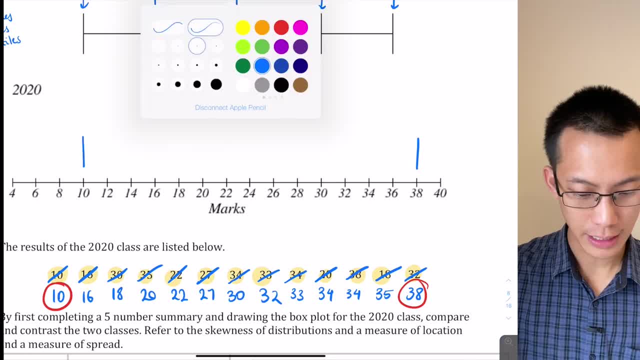 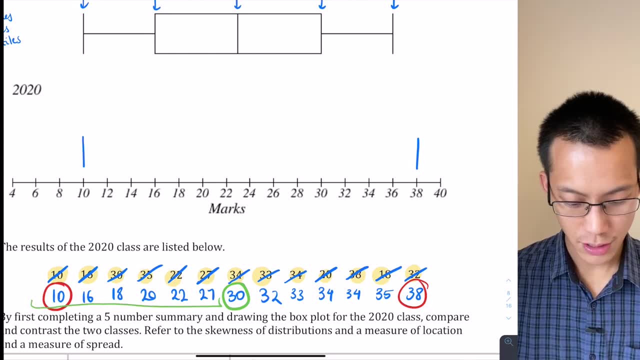 I've got 13 scores, then the middle score will be the seventh score. Let's find that on the list. The seventh score, by the looks of it, is going to be 30. And you can see there there's going to be. 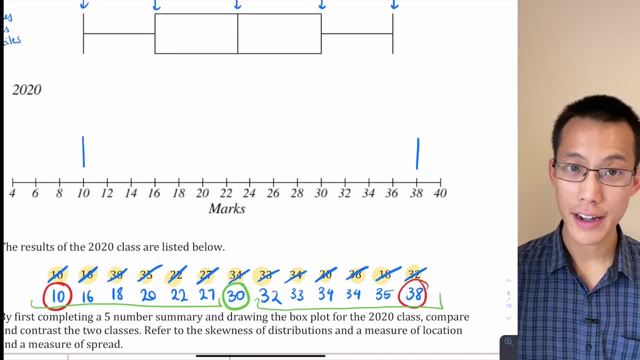 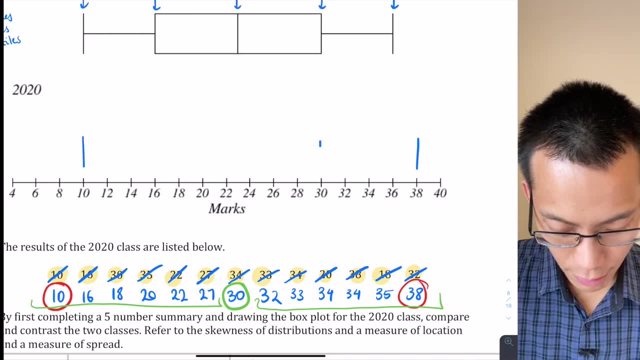 three left and six scores to the right. So I've divided it into two even groups. So I'm going to find 30.. That's going to be on my graph. here There's 30.. So there's going to be my median I. 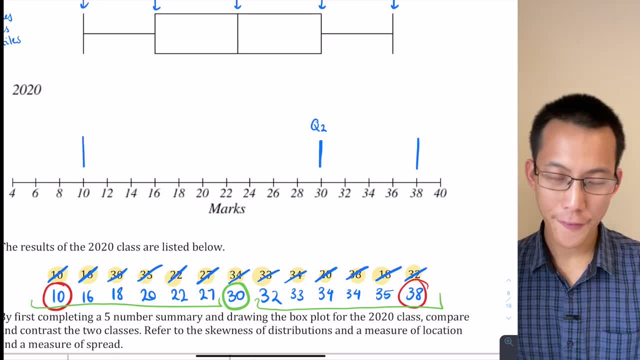 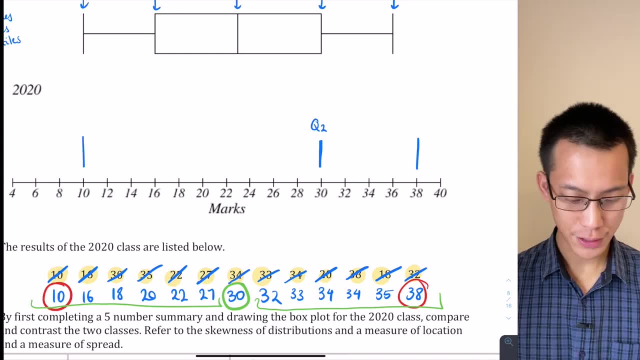 might even label that Q2, so I don't forget what it is. And then to find out my Q1, my lower quartile and my Q3, my upper quartile. I repeat that process, but for the data points that I have below. 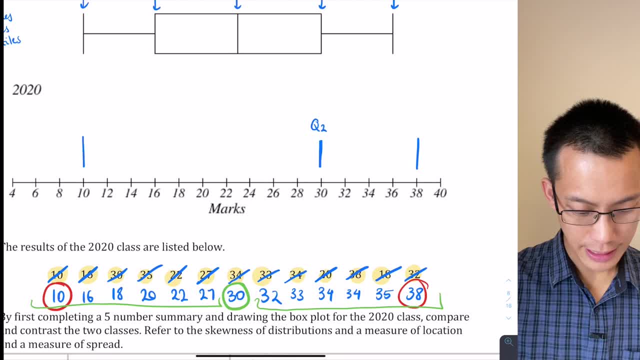 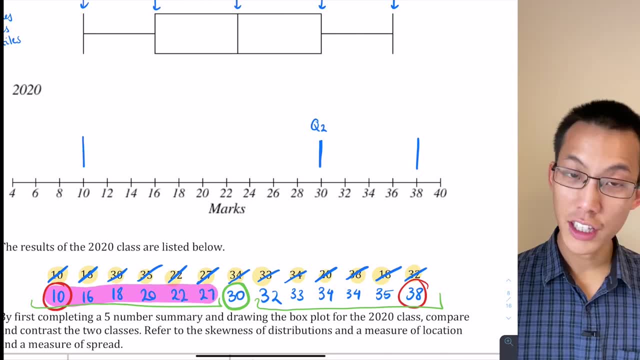 So when you have a look, you can see I've got. let's highlight it in another color that I haven't used yet. Let's use pink. So this is the lowest set of scores. Gee, that's really bright, isn't it? You can see, right? 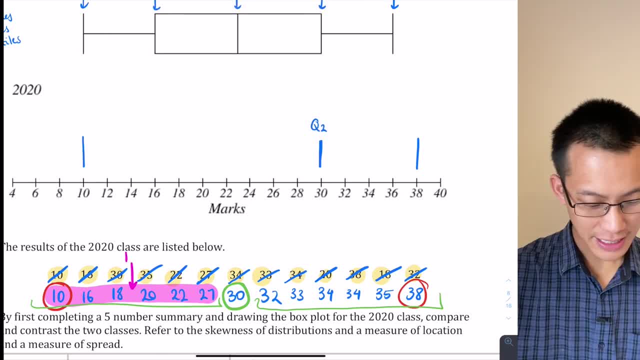 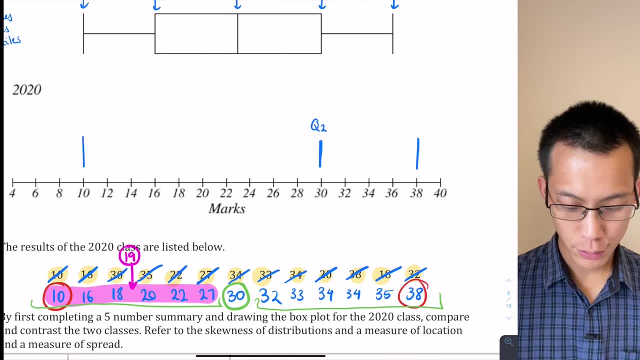 in the middle here between 18 and 20, is 19.. That's halfway in between. So 19 breaks that group into a group of three and another group of three And then, if you have a look at the data set on the 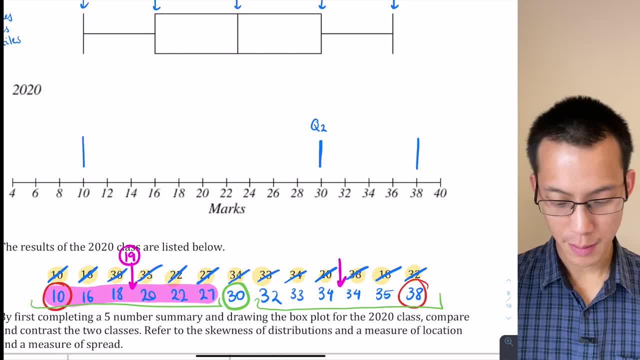 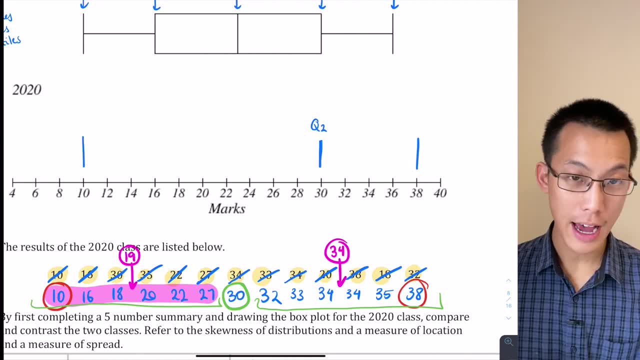 right, it would be in between these two scores which happened to be the same score. So 34 is going to be the upper quartile, If you like. it's the median of the top half and the medium of the bottom half. So now I find where those are on my vertical, my horizontal axis up. 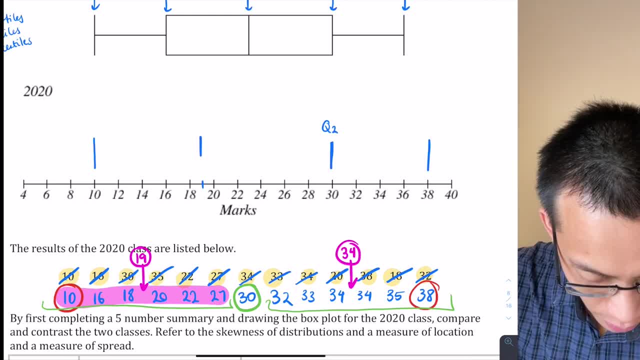 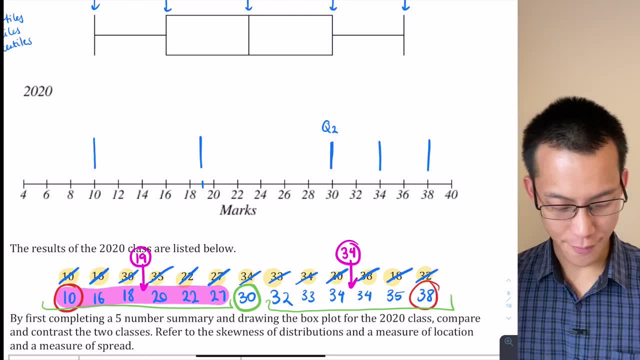 above here. So 19 is between 18 and 20.. So vertical line there. And then what did we say? 34. So here we go, All right, So I've done all five of my vertical lines. That's why we call it a five. 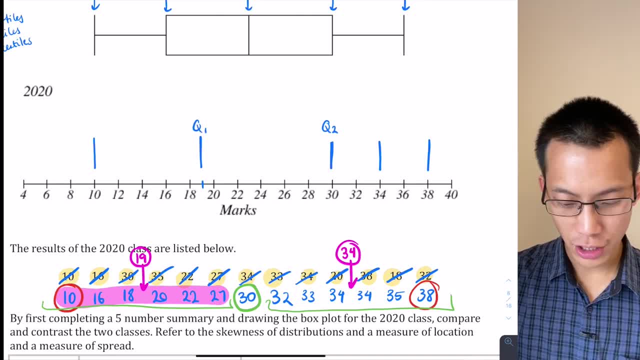 number summary: Q1,, Q2, and Q3, and then my minimum and my maximum, And now all I need to do is turn these lines into boxes and whiskers, So I'm just going to put this horizontal line in here. 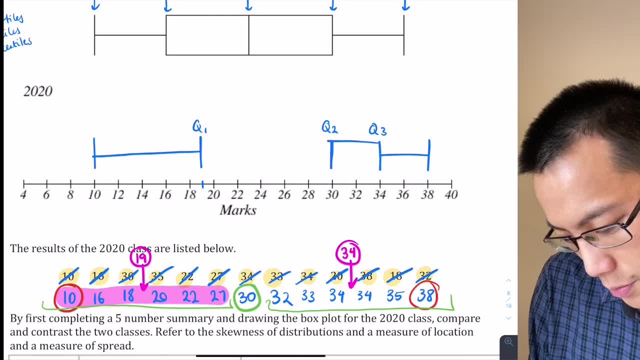 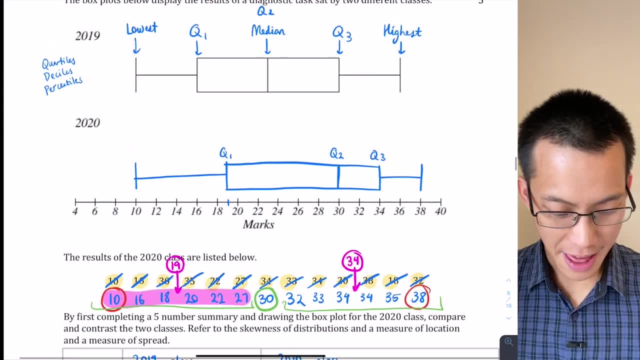 There's one whisker, There's the other one, And then here comes the box in the middle. It's not the neatest, but you get the idea. Okay, So I'm done. That is the box and whisker pot for 2020.. 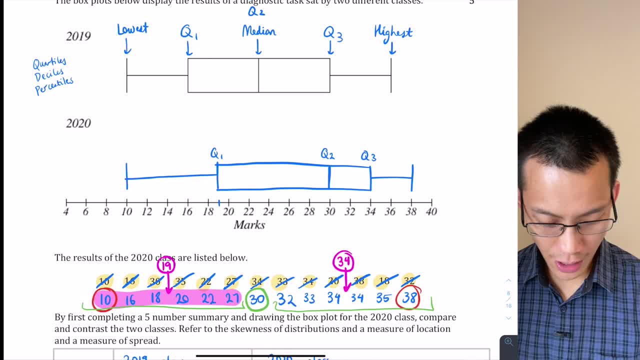 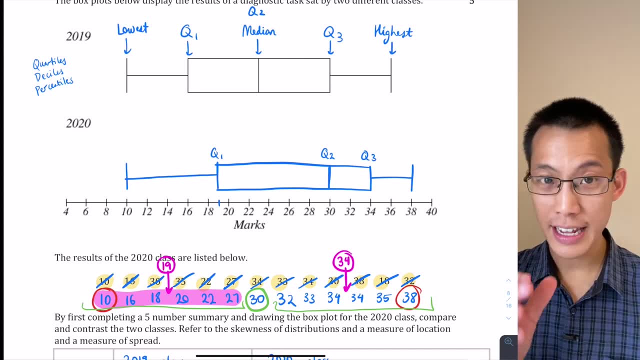 And now we're supposed to use that. You can see down the bottom to compare and contrast the two classes. Now this is really important. The question says refer to, and then it names a few things which, if you want to get full marks on this, 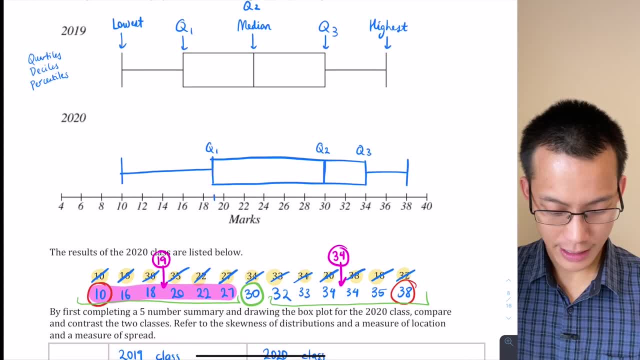 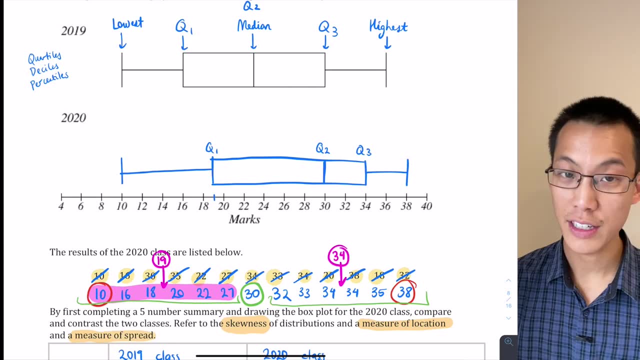 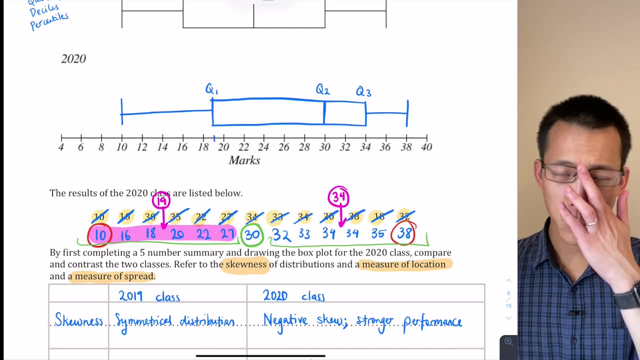 you want to identify those fairly deliberately. It says the skewness of the distributions, the measure of location and then the measure of spread. So let's talk about each one of those in turn. So skewness? Well, skewness talks about which way is the data leaning. 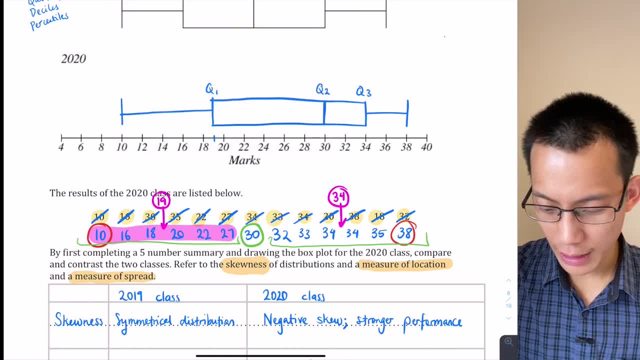 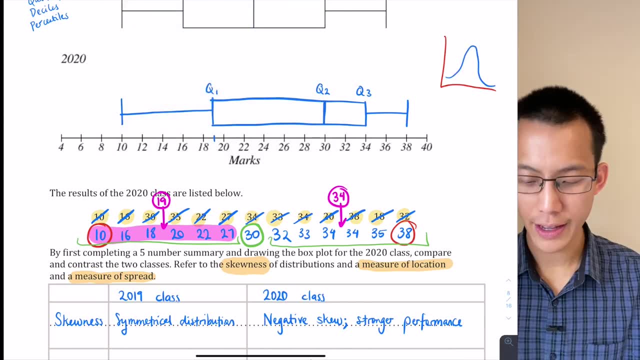 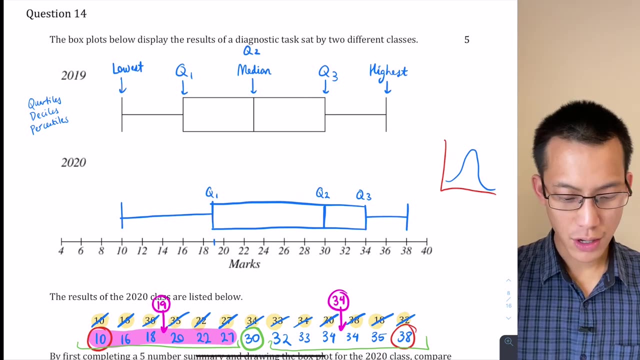 so I Will give you an example quickly here. What does it look like if you've got a sort of- you know- symmetrical data set? It's going to look like this: if you were doing a plot of it but on a box plot on a box and whisker plot, you can see what it means is that your lowest and your 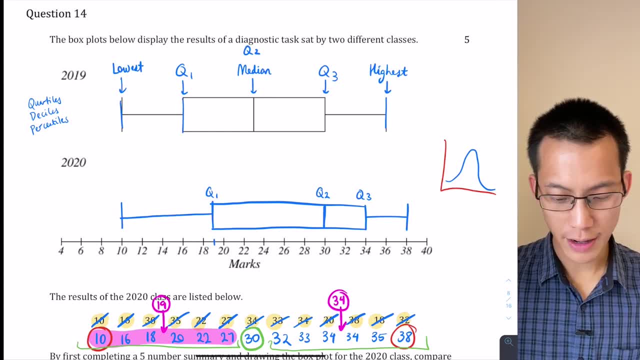 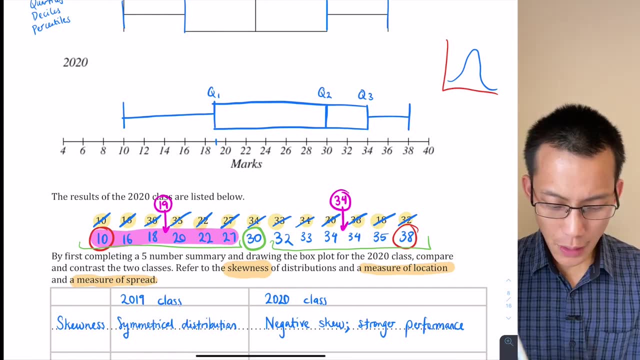 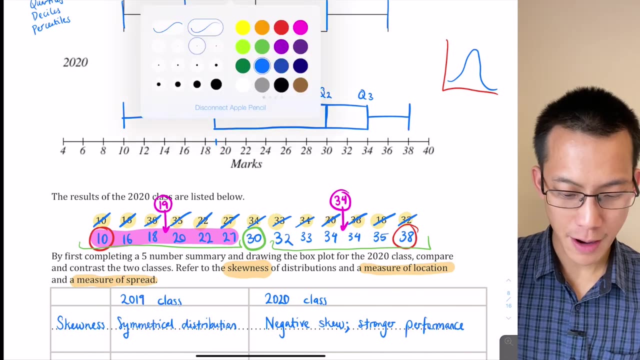 Highest are symmetrically positioned around q1 and q3.. So that's why you can see I've written that the 2019 class has a symmetrical distribution, but if you have a look at The 2020 class, there's a negative skew. Now, what does that mean? Well, if I go up here and again draw you an example, 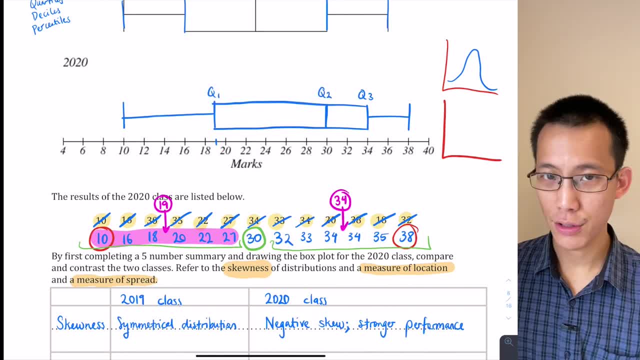 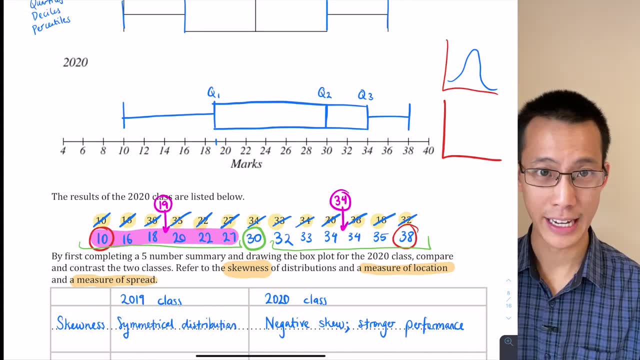 When you talk about skew, you've got positive skew, negative skew. I always remember it's a bit weird, It's a bit counterintuitive, because the skew refers to which direction is the tail going in. It's not where most of your scores are. It's where most of your scores aren't. 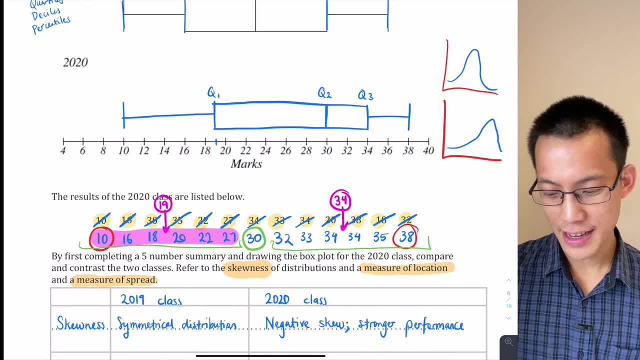 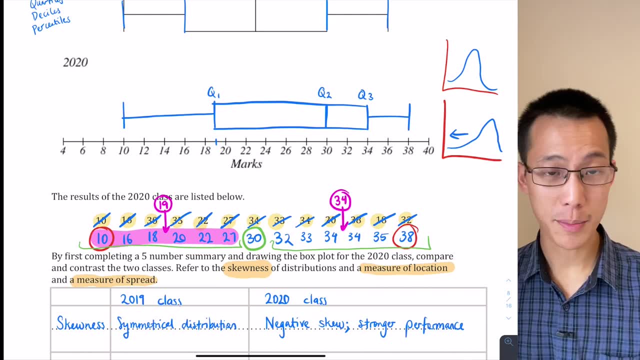 So a negative skew would be something like this: You can see I've got my tail pointing in the negative direction and that's what we have here. Most of the scores here are bunched up toward the top. You can see q2 and q3 are quite close to that upper value there. 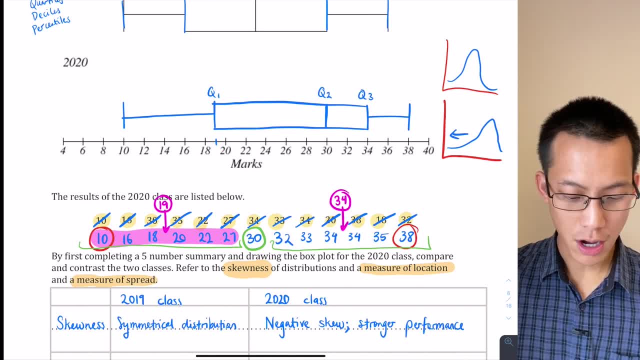 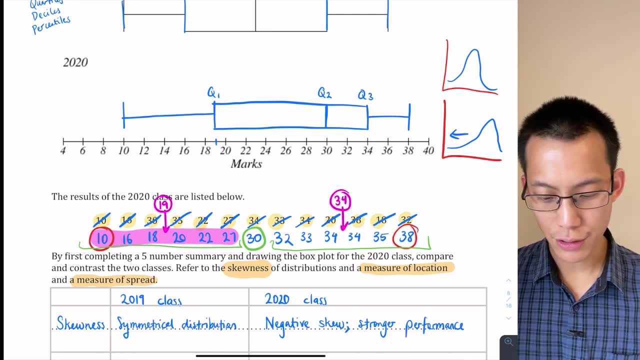 Whereas q1 and the lowest value over here on the right hand side they're quite spaced out. So you can see this gap here and this gap here are very large compared to these gaps over here. the larger those gaps are, the more spread out the students are, which indicates there are fewer students down the negative end. 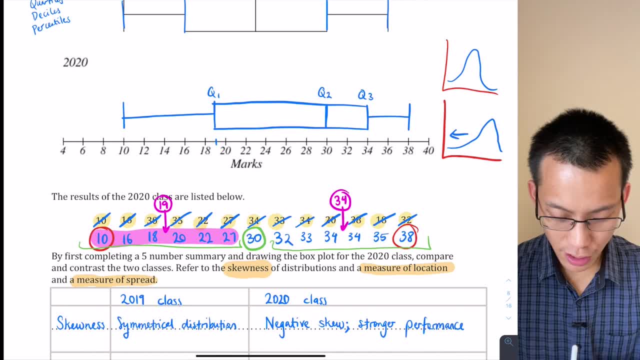 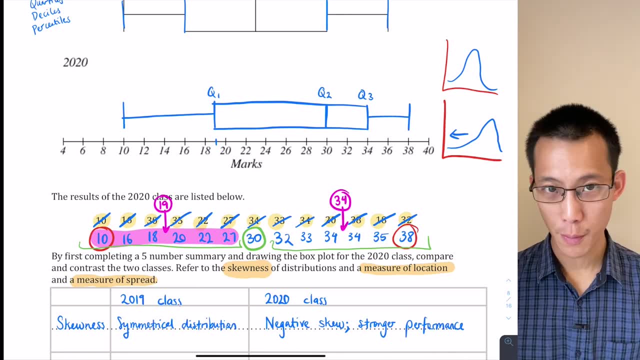 of the graph. So that's why I said there's a negative skew for the 2020 class as opposed to the symmetrical distribution. So that's a point of contrast: There's stronger performance for the 2020 class as compared to the 2019 class. I'm going to move down and now I'm going to talk. 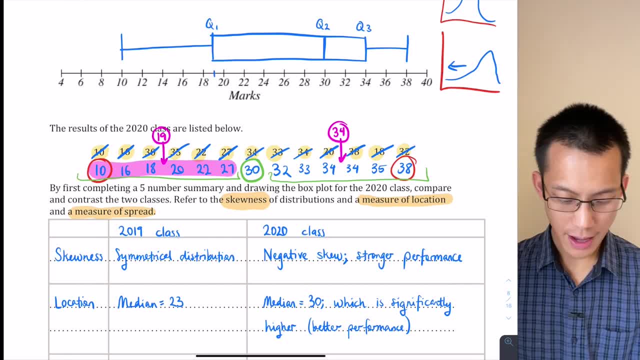 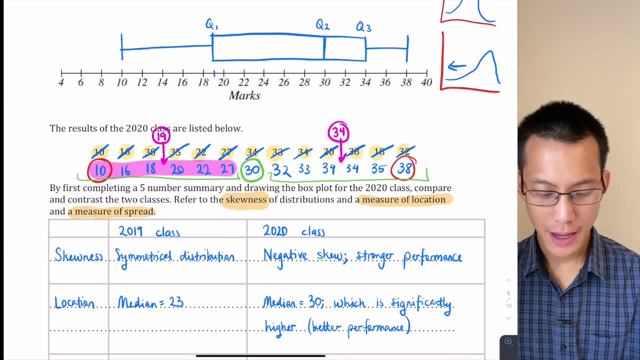 about a measure of location here. So what does location mean? That's talking about where, in terms of the marks, where are my marks actually positioned? Where are the students positioned? The only measures of location that we have really here are the median You might use mean. 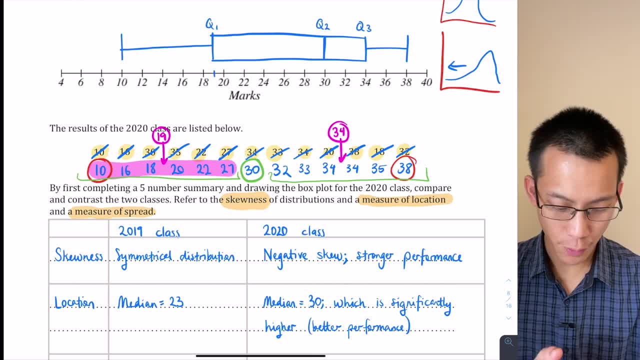 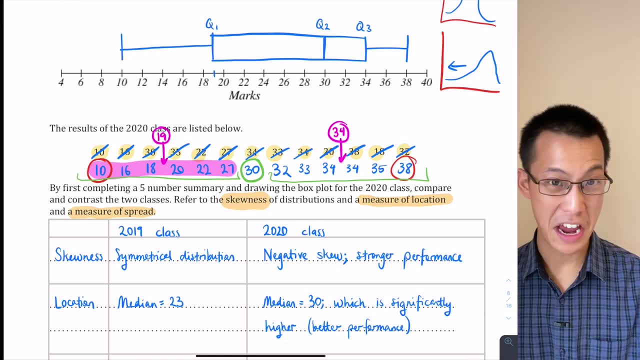 but we haven't got that calculated here. So the median for the 2019 class is 23 and the median for the 2020 class is 30 and that's way up like seven whole marks. So that's why I've written. 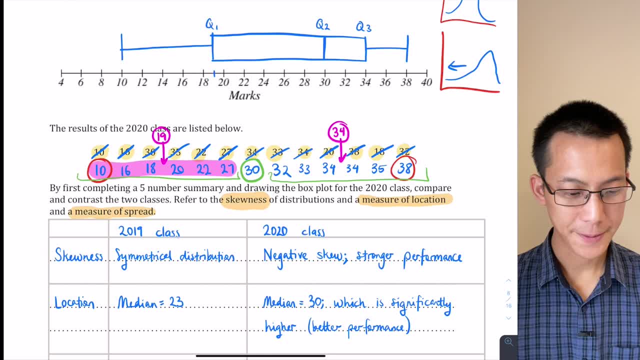 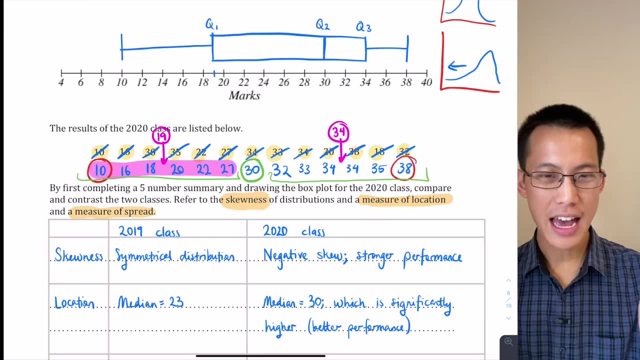 it's significantly higher and there's much better performance there. Then we go to measure of spread. Now you've got two different kinds of measure of spread here. You've got range and then you've got intercalation, So you've got intercalation and then you've got intercalation, So you've got. 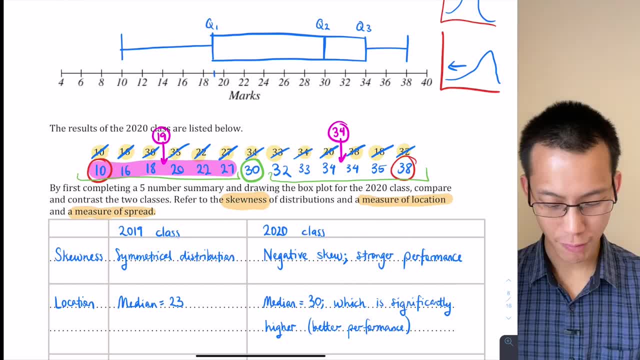 intercalation. So you've got intercalation, and then you've got intercalation. So you've got intercalation range, which is the difference between Q1 and Q3.. So I've written about both. You can calculate. 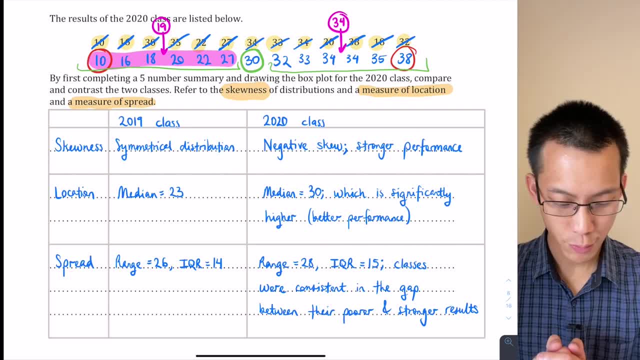 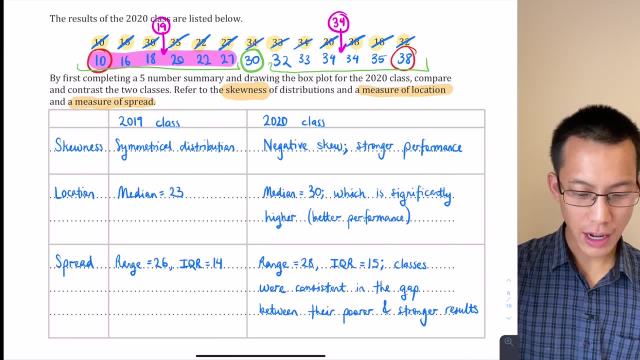 the range by doing top value, takeaway bottom value, which for the 2019 class is 26.. For the 2020 class, it's 28.. And then you do the interquartile range. Let me just write it in here. 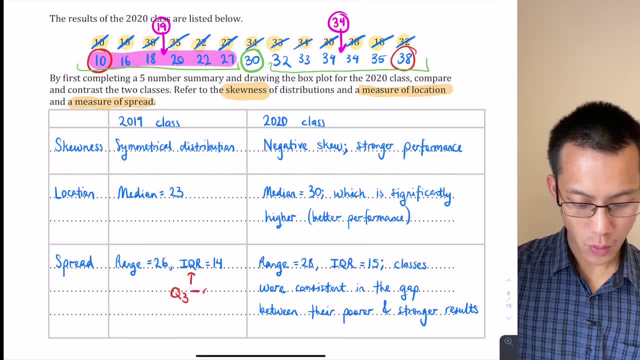 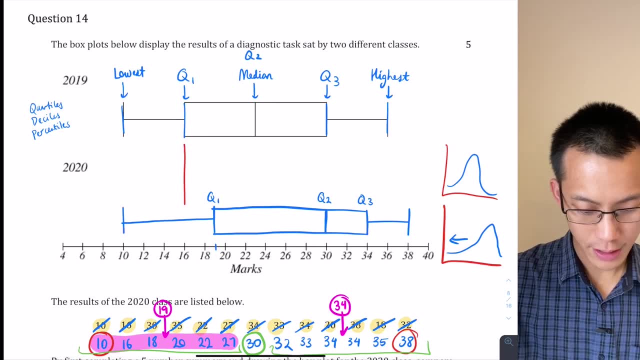 for you as Q3,, takeaway Q1.. So you can go ahead read from the graph above. It might help you if you go and say: oh, Q1,, where is that? It's going to be 16.. So you can go ahead and read from the. graph above. It might help you if you go and say: oh, Q1,, where is that? It's going to be 16.. So you can go ahead and read from the graph above. It might help you if you go and say: oh. 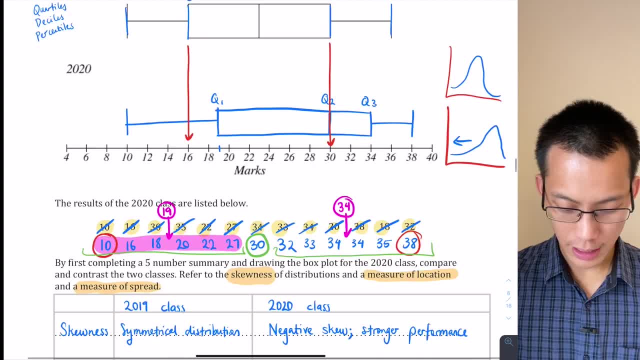 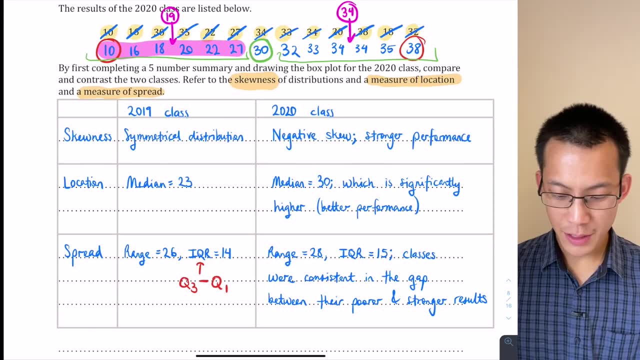 here, And then it is 30 over here. So 30, takeaway 16.. You can see where I got the 14 from. You go ahead and calculate it for 2020 as well And you get these results. Now, excuse me, It looks to me.